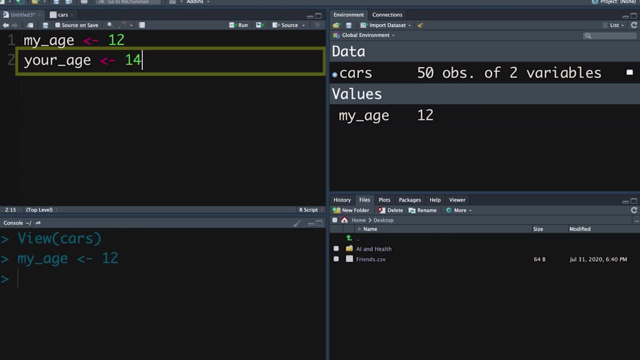 and we're going to say that your age is 14 and that pops into our environment over there. now how do we apply a function to these objects? the function sum, which is to add up, is the function right? and then we put brackets and we put the arguments of the function inside the brackets. 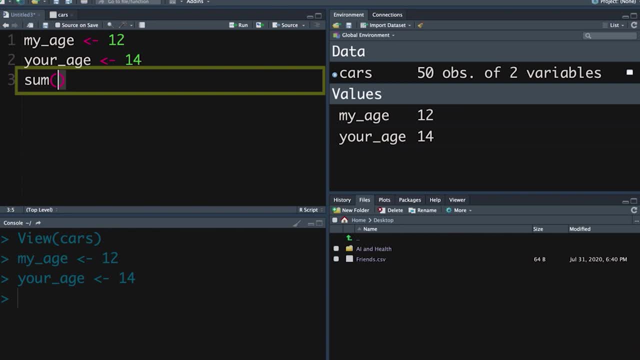 and the first argument is the function sum, which is the function sum, which is the function sum argument for any function is usually what objects that function should be applied to, and we're going to talk about other arguments in just a minute, but let's have a look. if we said we want the sum of my 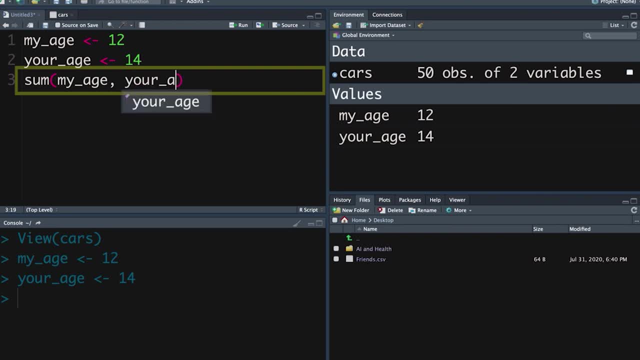 age and your age. uh, come on, enter and you can see down here in the console we can see it's added those up now. the most common object that we work with is a data frame, right, so there are all sorts of types and structures, but we're just going to deal with the common stuff now and we'll get more. 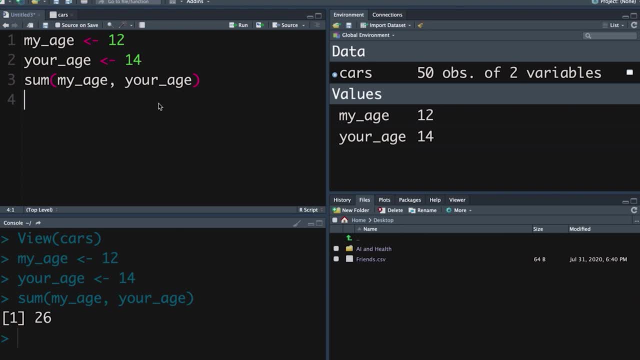 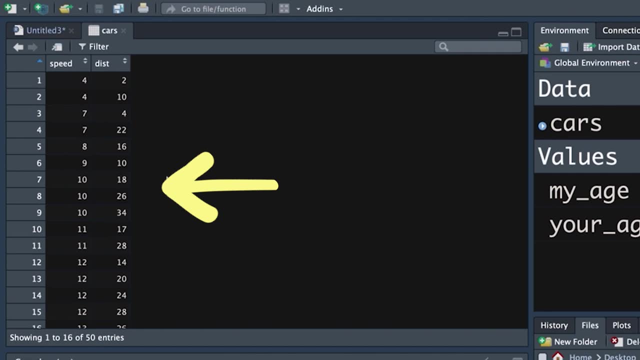 into the sort of more detailed uh variables that we're going to be talking about in a little bit, but let's have a look at cars right here. so if we click on cars, it's an object in our environment. that data frame pops up and we can see it here and a nice, neat and tidy, tidy data frame has got. 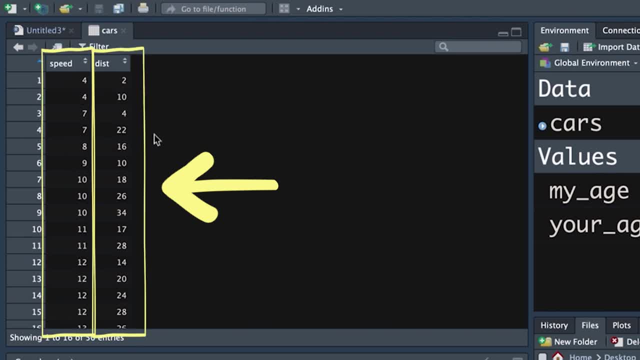 the variables as columns. so we've got speed and distance and each observation is a new row, right? so this is a typical format for a data frame, and we're going to look at how it is that we can apply functions to an object like this. so we might want to apply the function plot. okay, and plot is a nice. 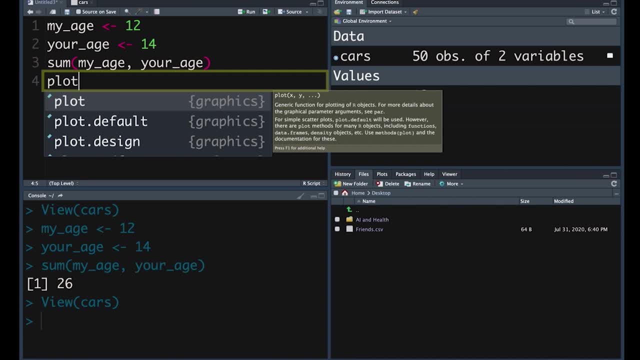 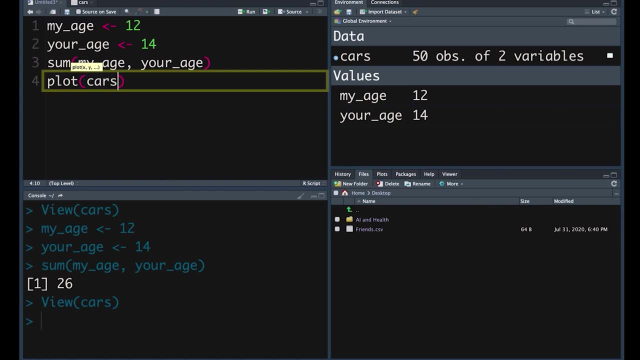 function because it r chooses the best kind of diagram that it can for any particular kind of data with plot and we want to apply the function plot to the data frame cars again. push command, enter and we can see down at the bottom on the right. it's created a plot of speed versus distance. 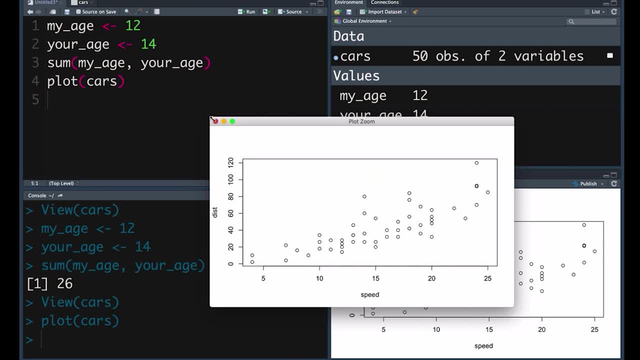 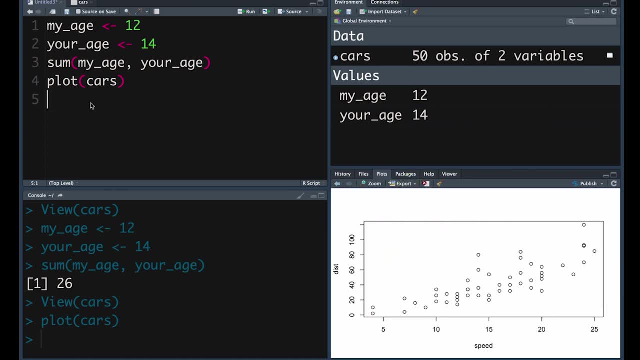 right there. we can zoom in and have a better look at that if we want to, and, of course, if we wanted to, we could export that as a pdf or an image. now we might want to apply a function to a part of the data frame, so not the entire data frame, but we might want to take one of the variables there. 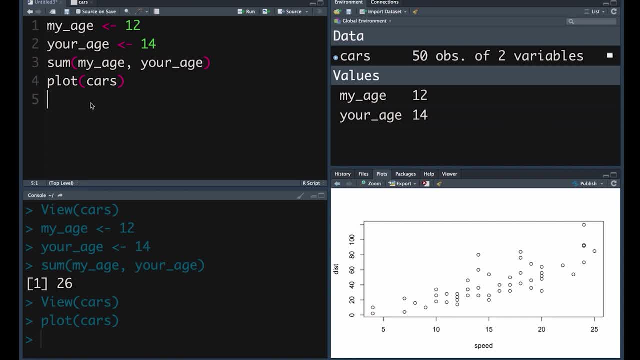 within, for example, speed, and we might want to apply a function to that. so if we've got a data frame, we've got multiple variables we can. let's say, for example, the function we want to use is histogram, or hist for short, open brackets. the data frame we want to use is cars, right and within that. 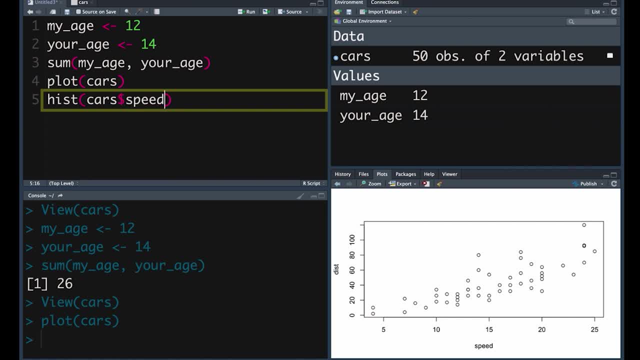 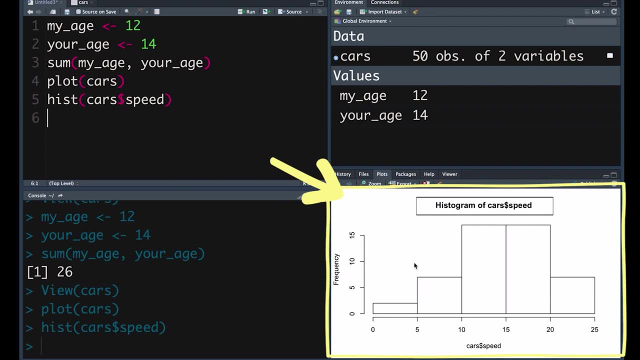 the variable we want to look at is speed, and if we push command enter we get a histogram of just the speed on the bottom, on the, at the bottom on the right over there. here's a neat little trick: if you use the function attach and you apply it to the object cars, command enter cars becomes attached. 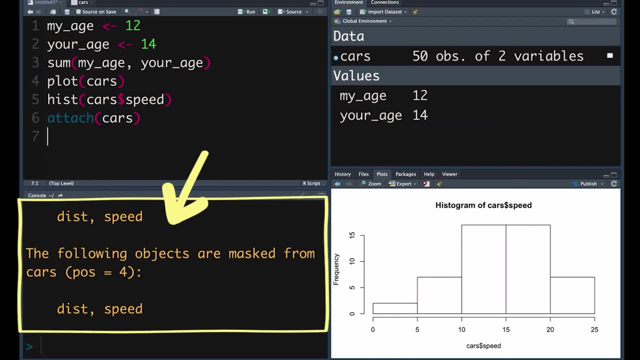 and so you don't need to use that little dollar sign to indicate which variable you want to use anymore. you can just type in the variable. so now, if we did hist, for example, and distance dist for distance, it would create a histogram of the distance without us needing to put cars. 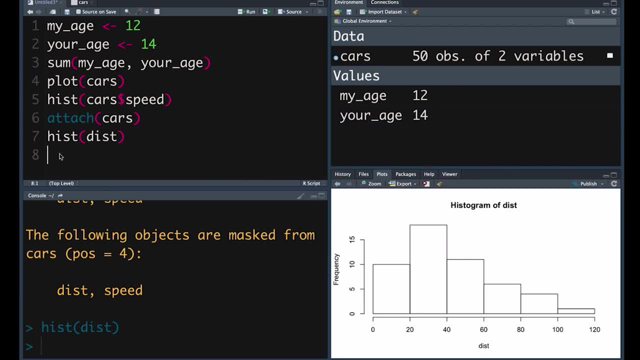 dollar sign dist. now there are hundreds and hundreds of different functions and, of course, as you install packages into r, you get even more. what i'm going to do quickly now is show you a couple of the functions that you can apply to objects. that will help you understand those objects. a 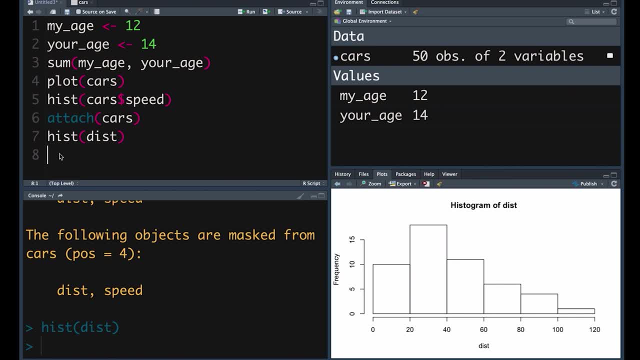 little better what the parameters and attributes of those objects are. so this is a great way to just sort of understand the nuts and bolts of the objects that you're working with and practice working with functions. first of all, you can do a summary of a particular data. 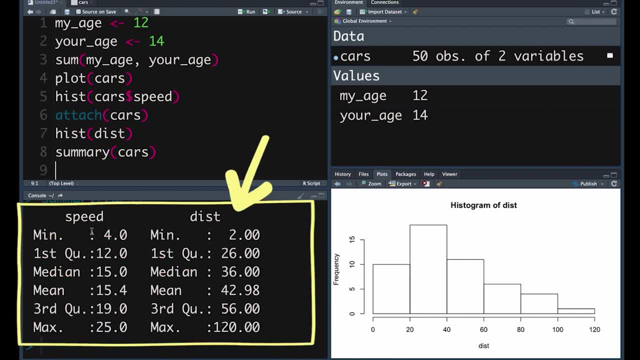 frame. if you push command enter, we get both variables, speed and distance, and it gives us basically- in this case they're both numeric variables, and so we get the minimum, the maximum, the interquartile range, the median and and and the mean for both of those variables, and of course we 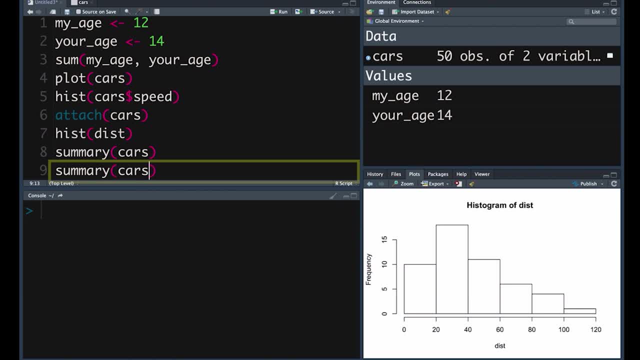 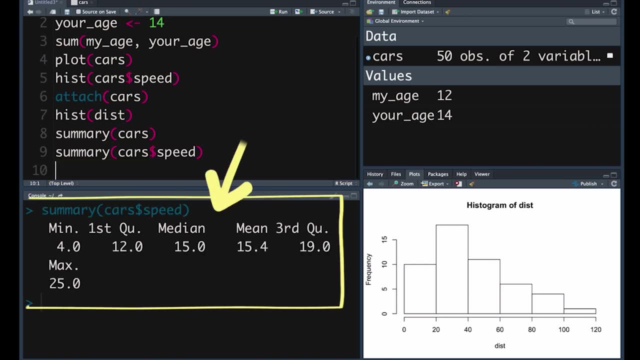 can ask for a summary of just one of the variables: right, cars, and i'm going to do the dollar sign and speed. but of course, because cars is attached, you don't need to do that. you could have just put in speed there, command enter and here we get a summary of just that particular variable. other: 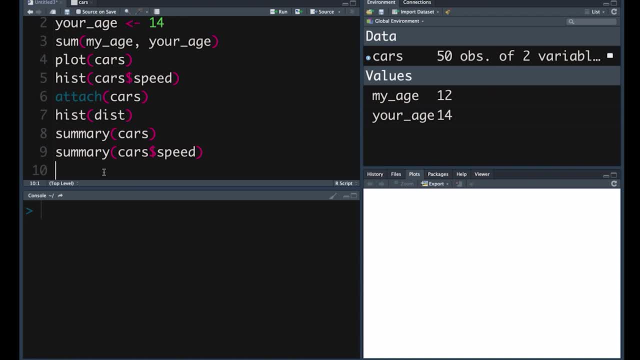 functions that are going to help you understand the attributes and the parameters of your data are class, for example, and we can put it in class cars, and that's going to tell us that cars is a data frame. class cars, dollar speed, and that's going to tell us that speed is a numeric variable. 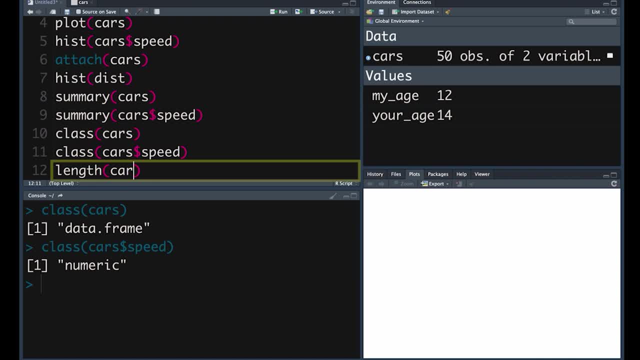 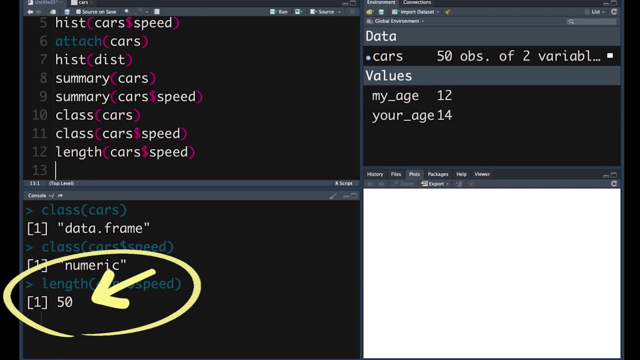 we can ask for the length of in the data frame, cars, the variable speed, and it's going to tell us that that has got 50 rows or 50 observations. we can also ask for how many unique very values there are. right, so things that like this is more. 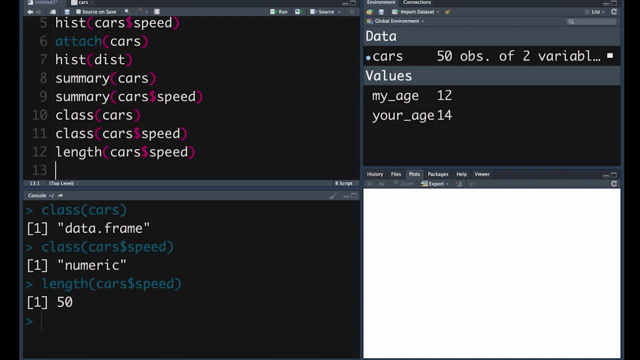 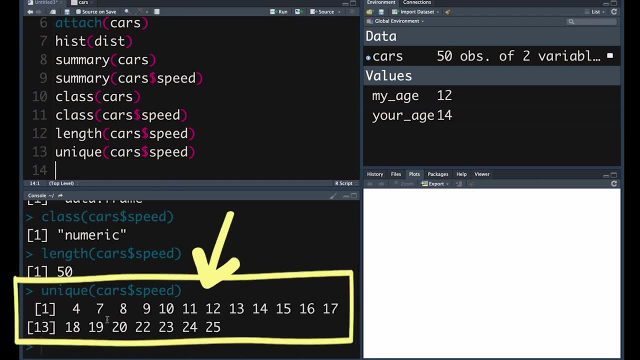 useful if you're dealing with, for example, a categorical variable, but let's do it anyway: unique speed, and it's going to say these are all the unique values that exist in that, in that particular variable. now you might want to get a sense of your data by looking at the first few rows or the last. 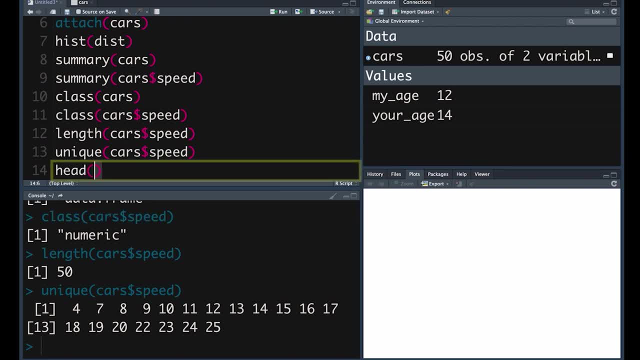 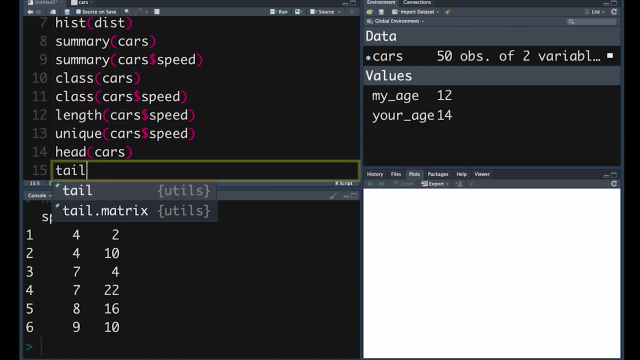 few rows of data so we can do head right, that'll give us the first few, it'll give us the first six rows, rather than I'll give you the actual effect: cars, and there we have the first six, six rows of data. and if we do the same tail cars- it'll give us the last six rows of data. if you 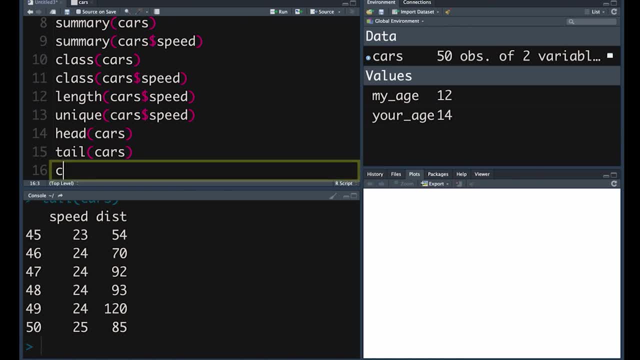 wanted R to extract out just a particular subset of your data. you can type in your object cars and then use the square brackets to tell it which subset you'd like now, and in the square bracket we're going to put a comma and I'm going to. I'm going to just do this one step at a time, for. 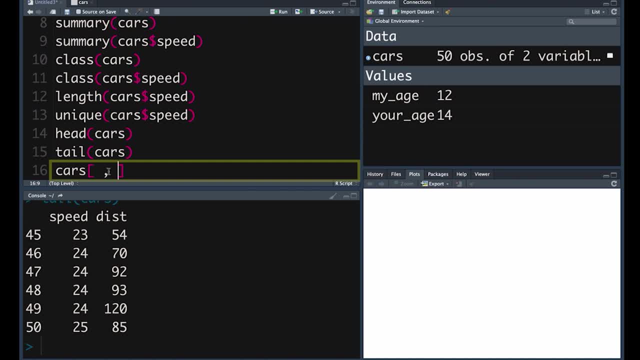 a comma that it saves. just come on pr4 because go ahead, I'm going to start with it because I'm just Microsoft Hauler. but, comma, you tell it what rows you want to look at and after the comma, you tell it what columns you want to look at, right? so if we wanted to look at row three to six and we wanted to look at 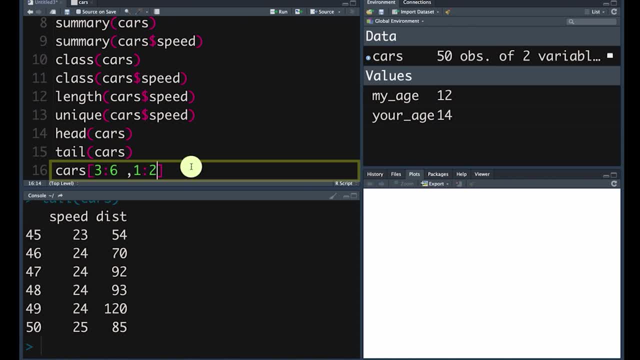 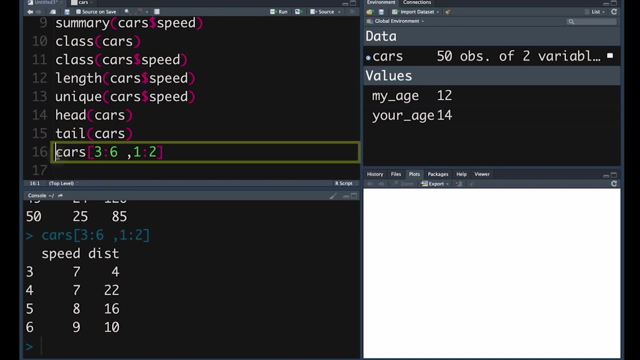 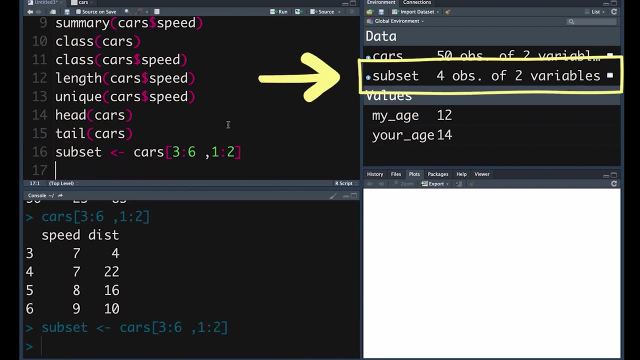 both columns, in this case one to two. it gives us that particular data frame, that particular subset, and of course we can actually assign that. we can call it subset if we wanted to. we could call it anything and voila, we've created a new little data frame or a new object called subset, and we can 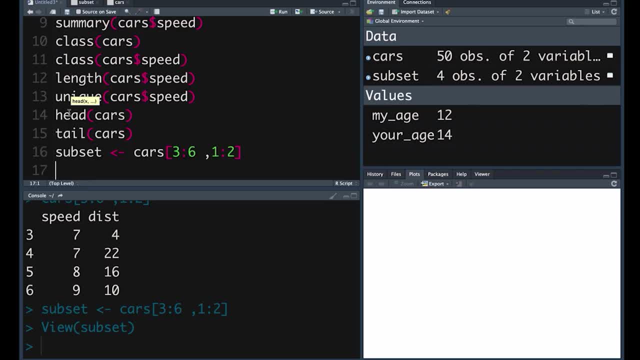 look at that right over there. now a little more about functions. right, functions have arguments. the first argument in a function is usually what data you're going to look at. but there are other arguments and i'm going to show you how that works right now. let's start off by saying: let's say we 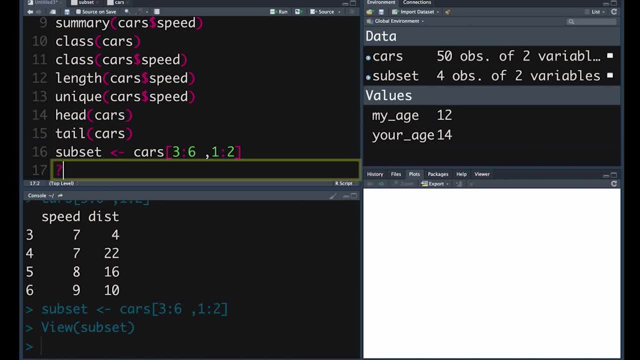 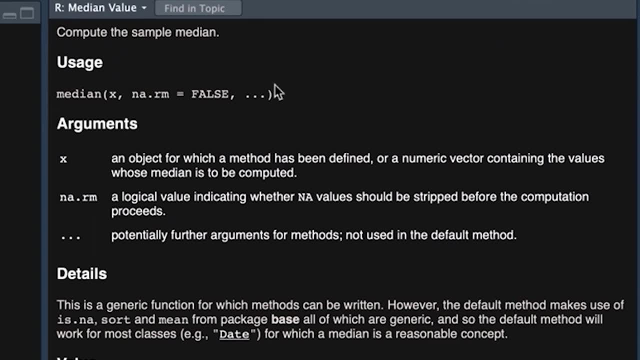 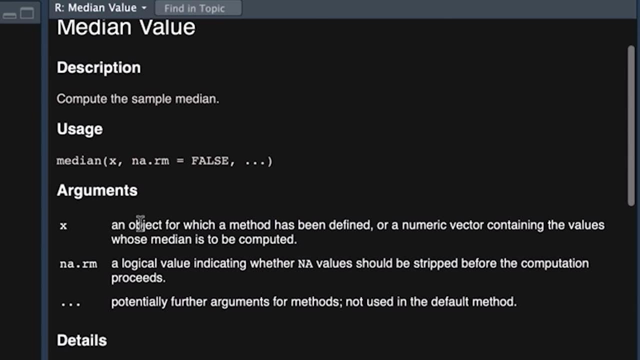 don't know much about a particular function like, let's say, the median. we can put a question mark and we type in the word median and in our help menu at the bottom on the right, we're going to see all of what we call the r documentation around this, and one of the things it tells us is: what are the arguments? what are? 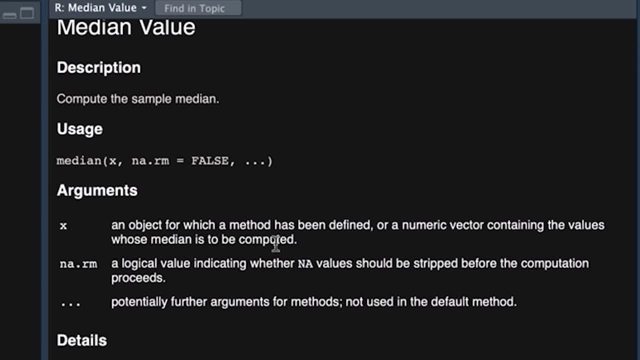 the things that need to go inside the brackets in order for this function to work. some of those arguments you need to input right. so, for example, you need to tell the function which data set or which object it needs to look at. but a lot of the a lot of the arguments are actually just set as: 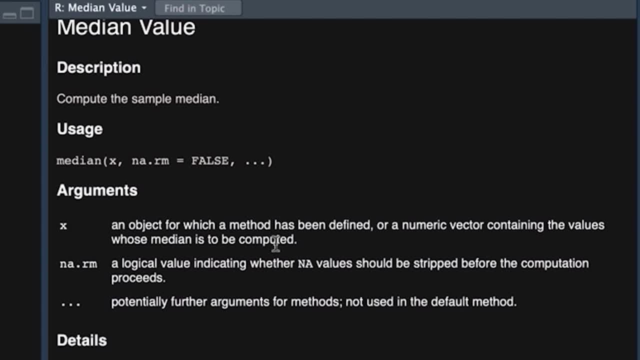 defaults and you don't need to do anything unless you want them to change right, and i'm going to show you how that works with this particular example. in the example of median, the narm, which is na, stands for not available or missing data and rm stands for remove. the narm argument is set by: 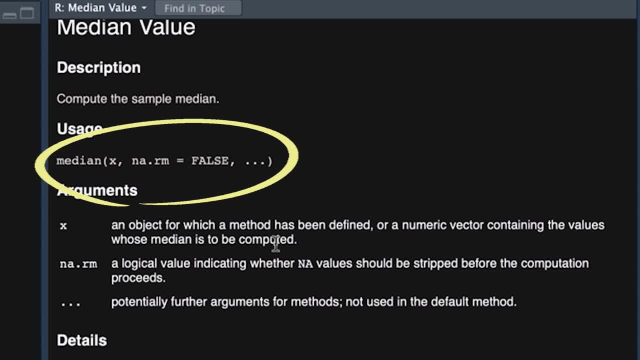 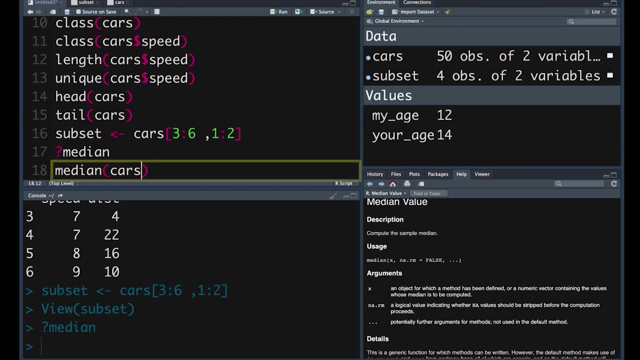 default to false and we can change that to true, and i'm going to show you how that works. okay, let's do that. so first i'm just going to show you how, if we use the function median, apply it to the object cars and the variable distance, in this case. 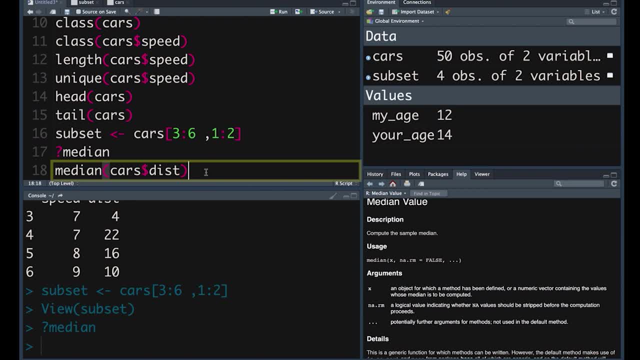 it'll give us and we don't need to put in that second argument. by the way, remember i said narm na remove argument is set by default to false. you don't have to put it in. r just assumes that it's false and in this case this data has no missing values. it doesn't really matter. so if we push. 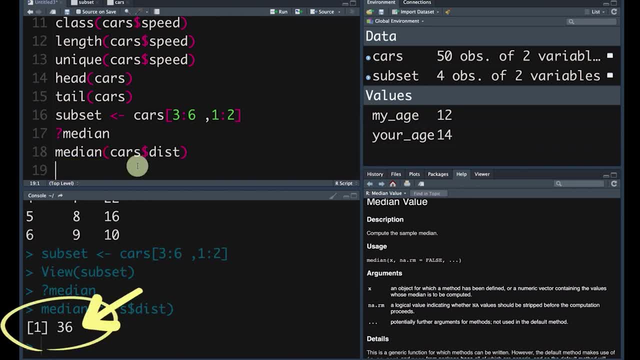 command enter. it just produces the median, in this case 36.. let's quickly create an object that does have missing values in it, and i'll show you how this particular argument works and how it is that we can change the value in an argument when we apply it. 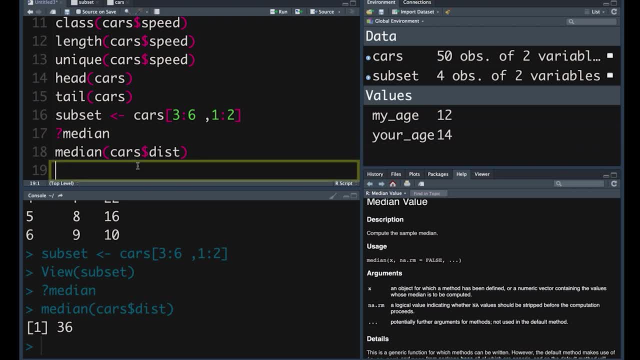 a function to an object, right? so let's create an object called new data. it's just going to be a single, it's just going to be a single vector. and if you want to put multiple values into a vector, what we can do is use a little c, which stands for concatenation. 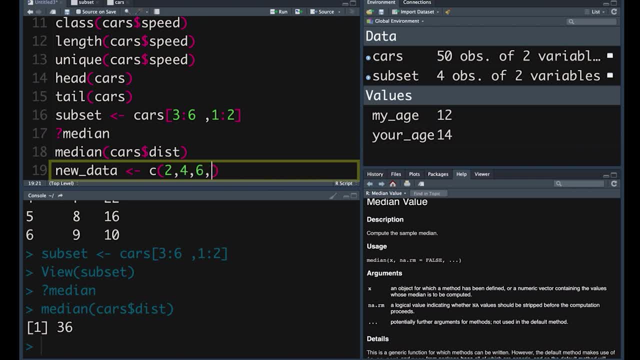 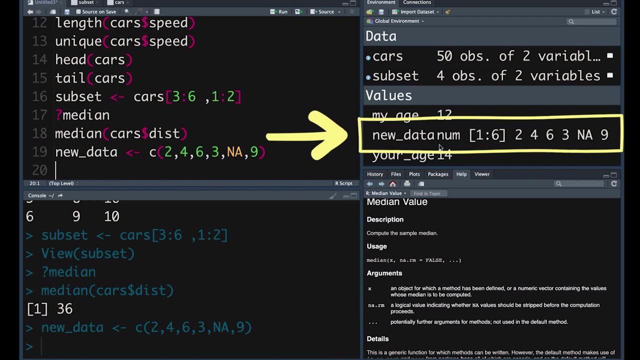 and we can say two, four, six, three. i'm going to put in na for not available, so there's a missing value there and we'll end off with nine, right, and you can have spaces between those, it doesn't really matter, it's just going to be a new vector, so we can just move it around and we'll see what it does. 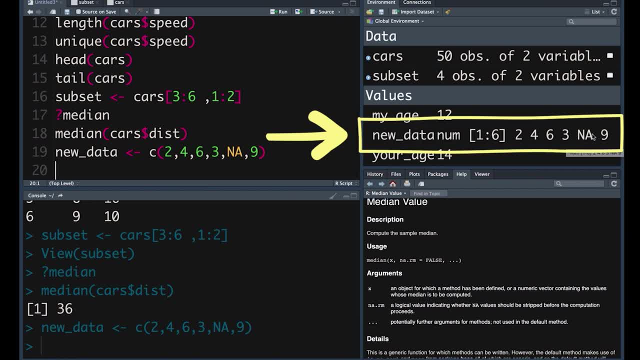 so we're going to create a new object called new data and we're going to call it r and we're going to put in a new data right command enter. now we've got a new object here called new data. it's numeric and there are the values and we can see the missing value is right there. 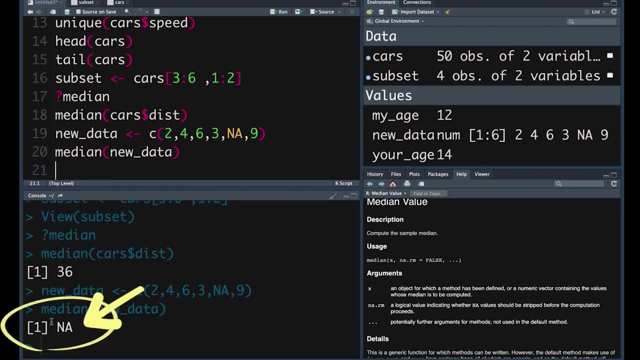 if we apply the function median to that object- new data because there's a missing value- r is giving us na. it cannot calculate the median because there's a to that second argument. So comma NA remove is equal to true, In other words remove missing values. 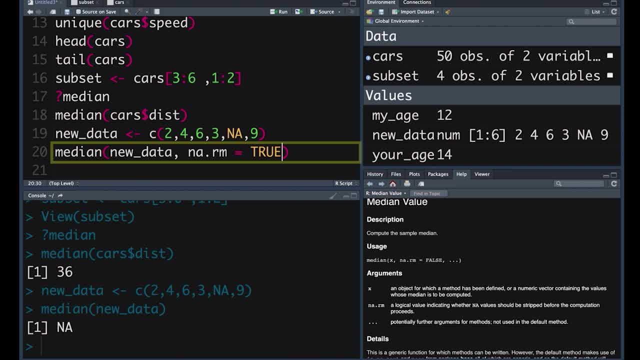 The NA remove feature of this function is set to true, It'll remove missing values and then try and calculate the mean. And now if we push Command Enter, voila, we get the median value Right. I hope that was useful. Just to summarize: we've got objects right. 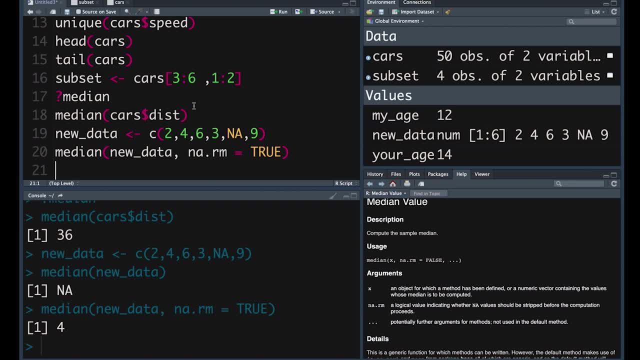 And objects have got different structures. We talked about the one structure, which is a data frame. that's the most common structure And within that there are variables. Variables have got different types right: There's numeric, there's categorical, et cetera, et cetera. 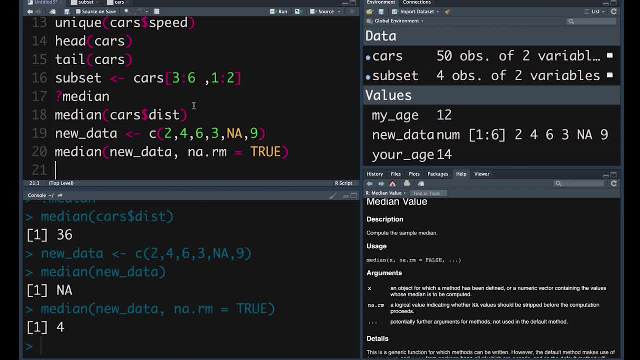 We're gonna talk more about that in another video. We apply functions to those objects. Those functions are instructions are to do to those objects, to that data. But sometimes there are additional arguments that we need to put in to give more specific instructions. 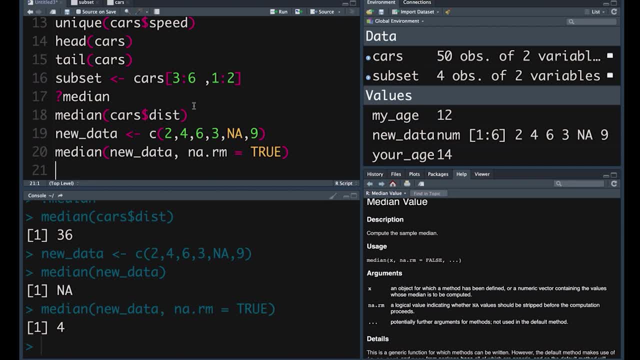 as to how it is that that function should be applied to that object. right? I hope you found that useful. Take care. 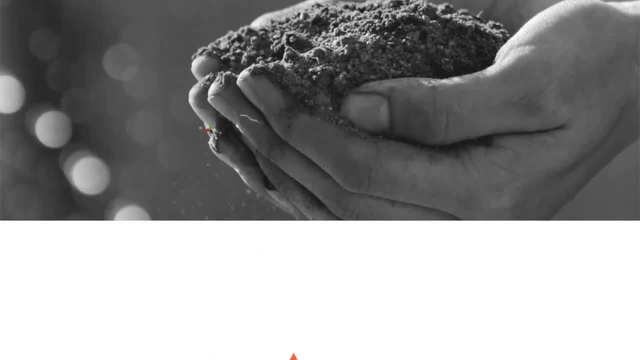 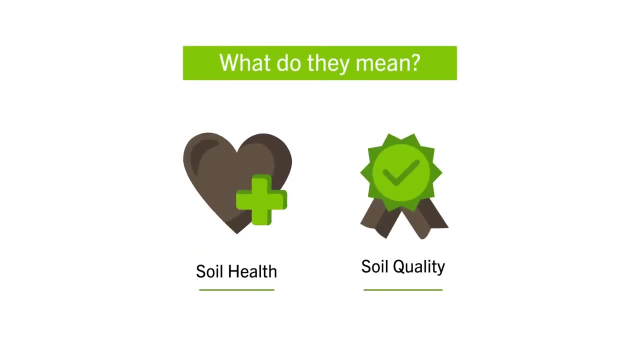 Today we're going to answer the question: what does soil health and soil quality mean? These are two terms that are often used together, and we are going to distinguish between the two and define exactly how they relate to your farm. These two terms are often used synonymously and